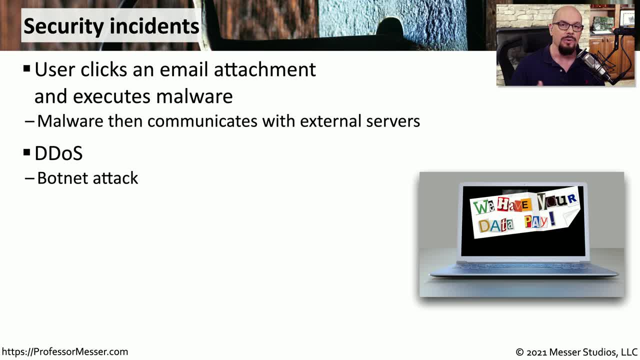 Or maybe you're dealing with a distributed denial of service attack with botnets that are overloading your internet connection. Or maybe information that was stored confidentially on your servers has now somehow made its way onto public servers on the internet, And sometimes the thief contacts you. 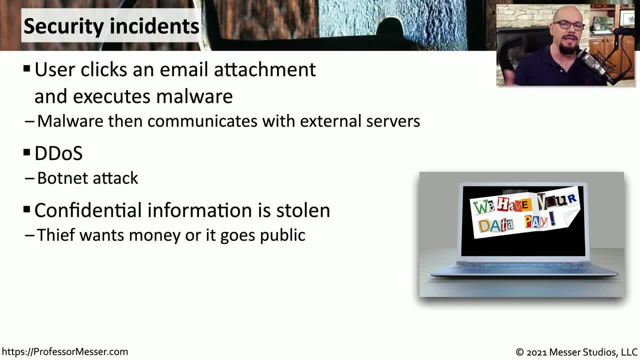 before making it public, to see if you'd like to pay a little money to keep it away from the public's eyes. Or you could have a user installing peer-to-peer software inside of your organization and effectively opening up all of your systems to access from the outside. 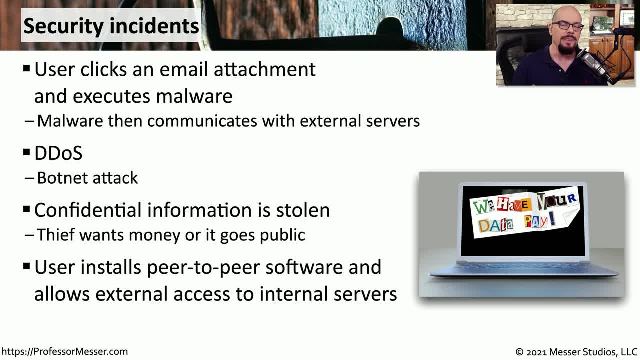 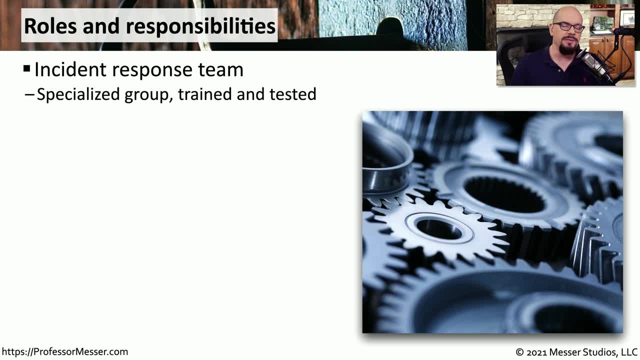 Each one of these security incidents are very different, but they all require some type of response by the security professionals in your organization. These types of incidents are often responded to by your incident response team. This is a group of people that have been specifically trained. 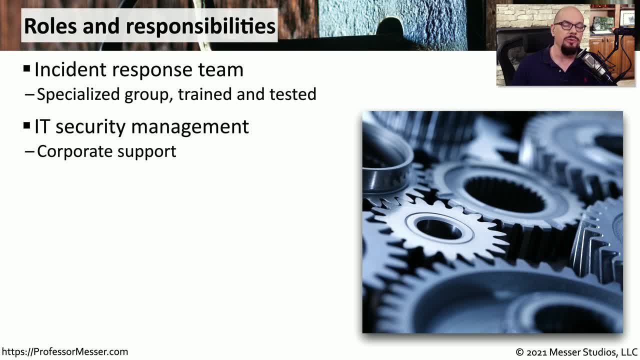 to deal with these types of circumstances. This might include the IT management team for your security department, so you have corporate support. It could have compliance officers that are responsible for making sure that all of the data is compliant with all of the rules and regulations. 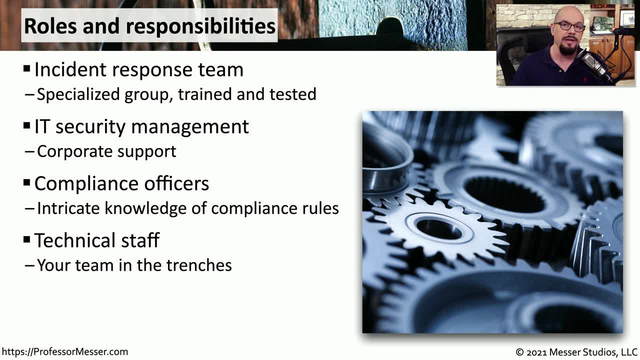 followed by your organization. You'll, of course, need technical staff to help troubleshoot and resolve these types of problems, And there may be users in your community that can help with these situations as well. This is certainly not a comprehensive list. You could have management within the organization. 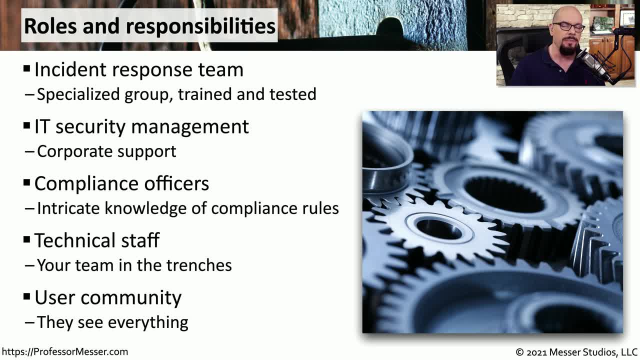 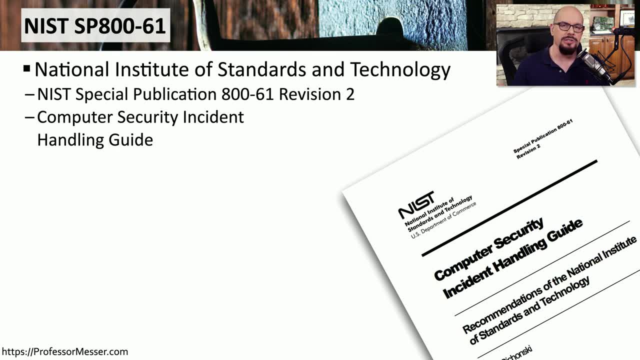 public relations, applications developers and other people who would be critical for responding to these types of incidents. NIST, NIST, NIST, NIST- The National Institute of Standards and Technology here in the US- have created a document that can help you understand the process. you'd. 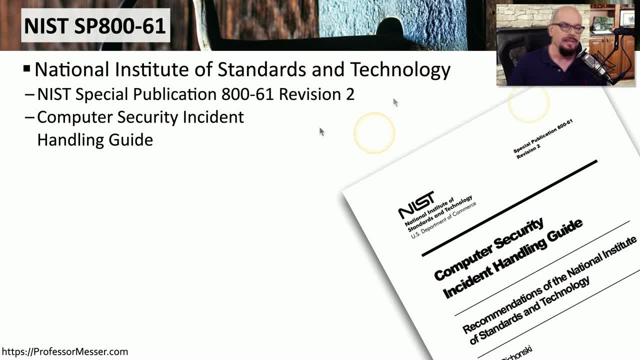 go through to handle these types of security incidents. This is NIST Special Publication 800-61, Revision 2, which is titled Computer Security Incident Handling Guide. This gives you information about the entire lifecycle when you're handling a security incident. This includes preparation, detection and analysis. 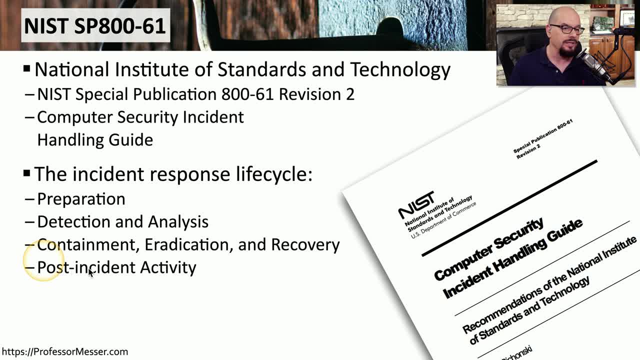 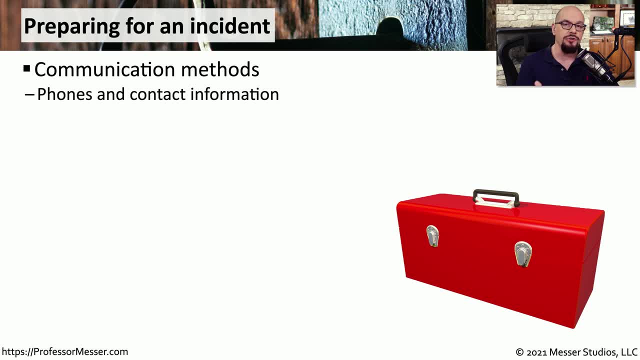 containment, Eradication and recovery and, lastly, your post-incident activity. The key to handling a security incident properly is to make sure you're well-prepared. There needs to be all of the right people and processes in place so you know exactly what. 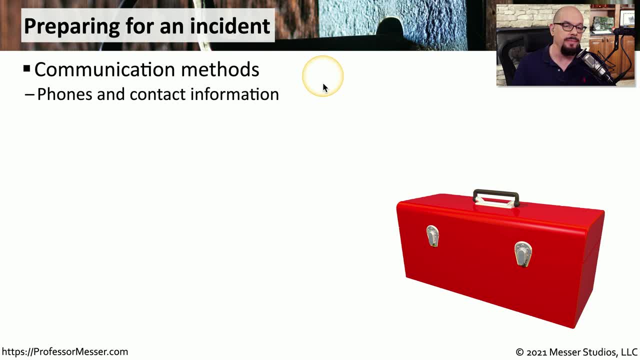 to do when the incident occurs. This would include communication methods, which will document exactly who should be contacted and how they should be contacted. This would also include your hardware and software tools, so you know exactly How to respond to these problems, store and capture data. that's important. 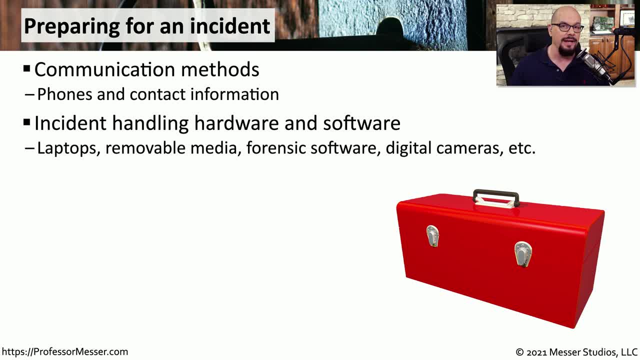 and be able to have information that you might want to use later on as evidence. There will also be a need to have documentation of the organization's network, understand exactly where data may be located, And once you have created and stored some of this evidence, 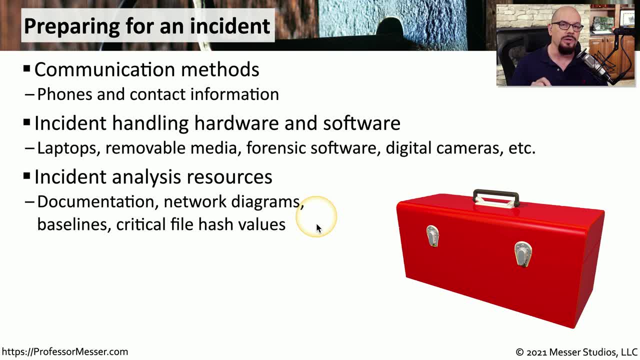 you may want to create hash values of that information so that you can be sure that none of that information changes. You also want to prepare for the mitigation process, so you want to be sure That your planning includes a clean operating system and application images. 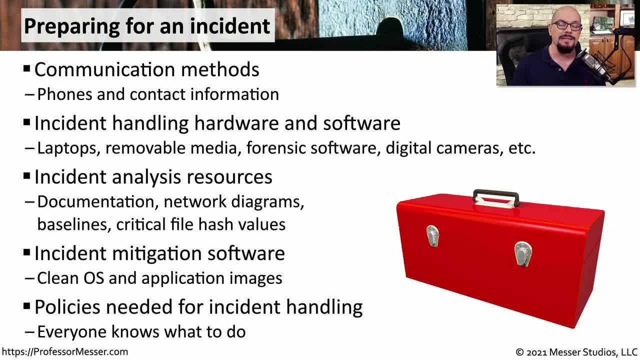 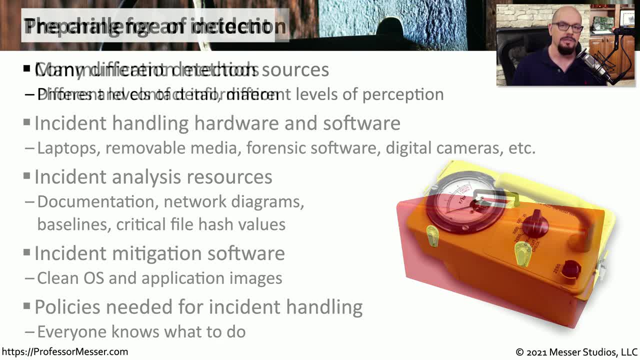 And lastly, and probably most importantly, we need policies and procedures so that everyone knows exactly what they should be doing when a security incident occurs. To be able to respond to a security incident, you have to know that the security incident has occurred. 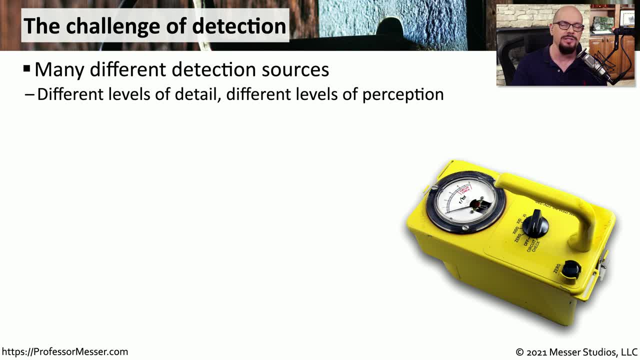 And there are many different ways to monitor and identify these security incidents. This is an ongoing challenge because we receive so many different types of attacks All the time, every day, And there are always security tools we have in place that will prevent the majority. 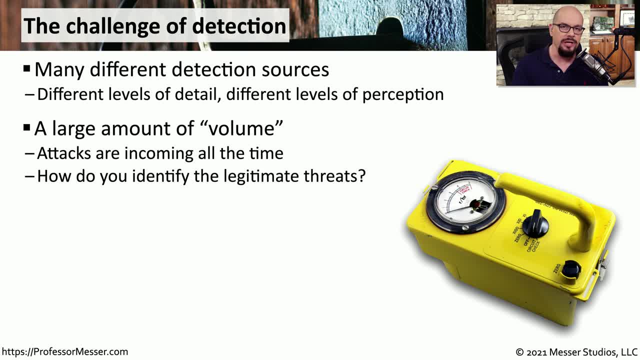 of these types of attacks, But how do you identify the legitimate threats and know if a particular incident has occurred? These security incidents often include many different devices, many different operating systems, And you often need someone who's very knowledgeable in order to understand exactly when an incident might have occurred. 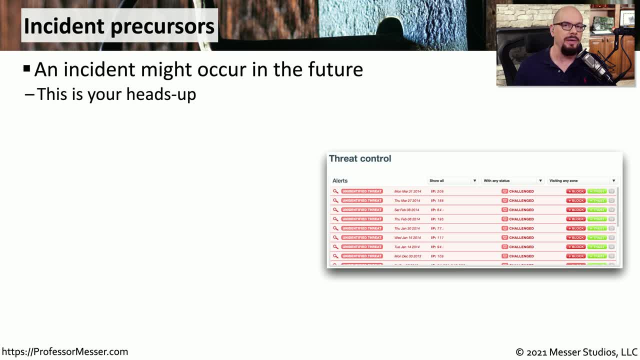 Sometimes we can be informed when the potential for an incident may have increased. These precursors give us a little bit of a heads up, or at least help us to predict where particular areas of the network may receive a security breach. For example, we may look through a web server log. 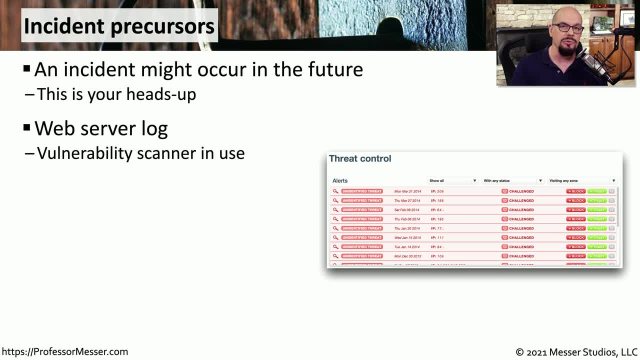 and see that someone was using a vulnerability assessment tool to try to identify any open or known vulnerabilities on that server. Or it may be that announcement day where we receive a list of vulnerabilities in Microsoft operating system. Or it may be that announcement day where we receive a list of vulnerabilities. 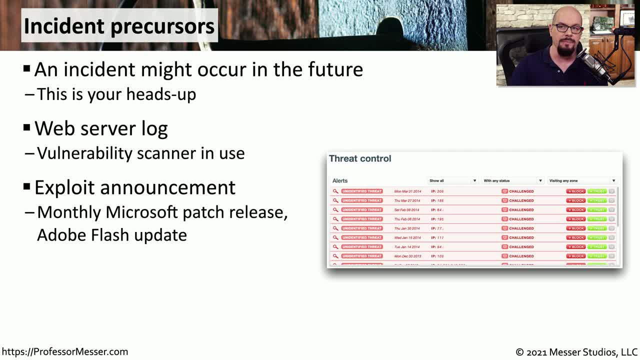 on that server And we can look at the security systems or Adobe Flash that tell us that we need to update those systems to avoid any type of vulnerability. Or there might be direct emails, Twitter messages or Facebook posts from a hacking group that tells you. 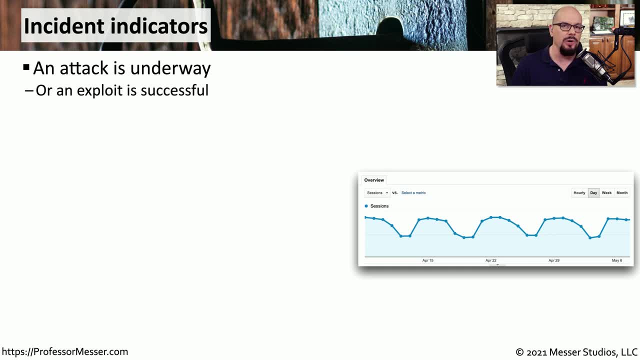 that they're going to try to attack your network. This means that we'll need to monitor our systems and see if we can identify cases where a particular security incident might have occurred. For example, we might find that our intrusion prevention system has a buffer overflow attack against our system. 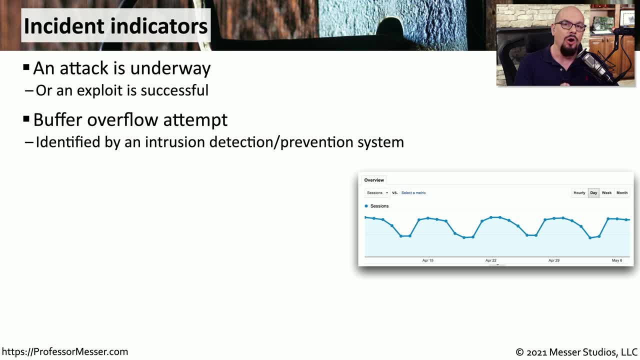 And it can tell us whether that particular attack was successful or whether it was stopped by the IPS. We might also have alerts and alarms that come from our anti-malware or anti-virus systems that can tell us if a particular piece of malicious software. 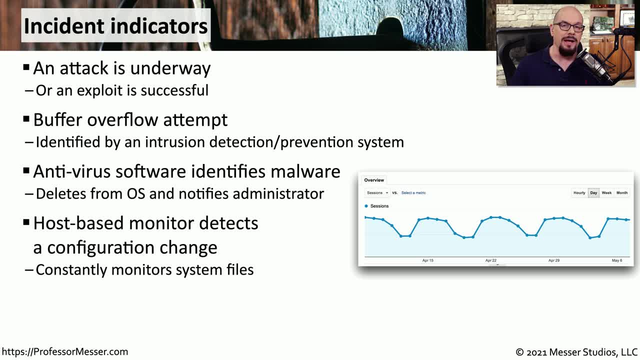 is running on a device. We can also have messages from our file integrity monitoring systems that will be able to tell us if any of the critical operating system files on our servers have been changed or modified. And if we're monitoring network traffic, we may be able to tell if there are differences in the traffic. 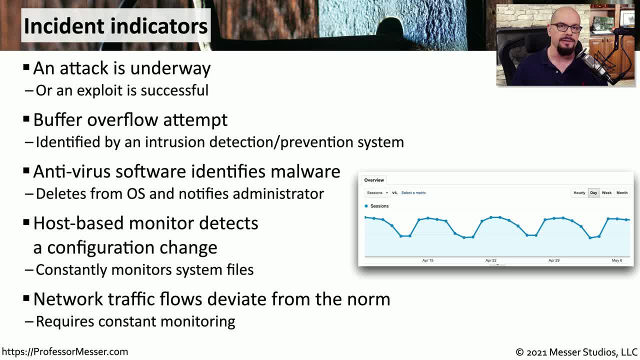 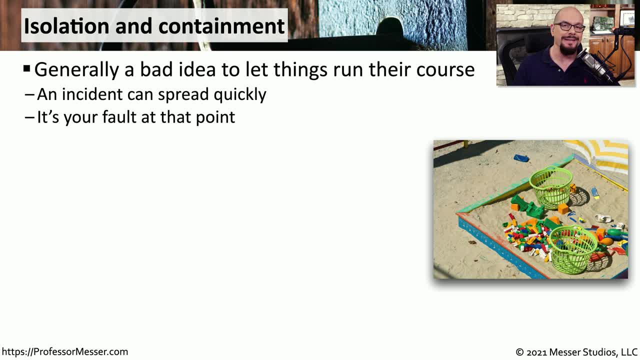 as compared to what might be normal on that particular segment. If you do find that there is malicious software or some type of breach, one of the best things you can do is isolate and contain that particular security incident. You would never want to leave it running just. 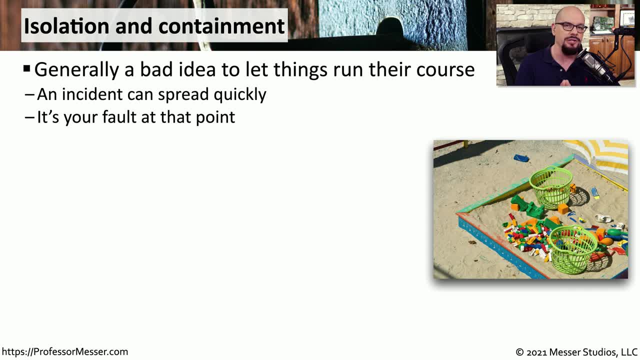 to see what it does, because nothing good can ever come from a situation like that. Instead, we might want to take that malicious software and run it in a sandbox. This would be an isolated operating system that is specifically designed to run software and see what the results of running that software might be. 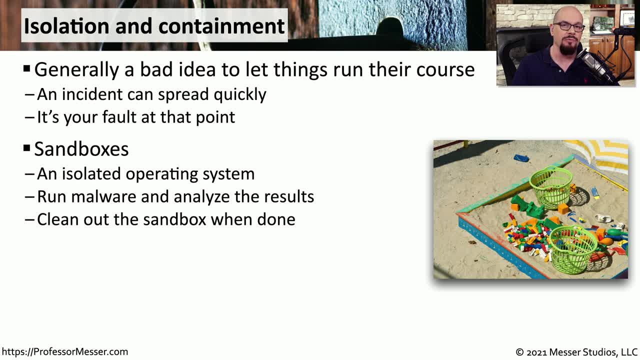 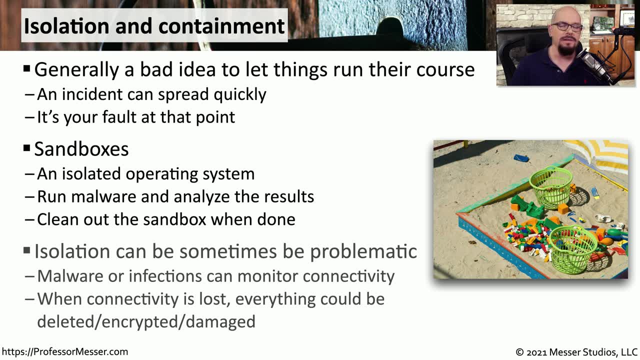 This is also an environment that can be completely deleted after performing your analysis so that you can be assured that that malware is not going to get outside of your sandbox. But even a sandbox doesn't provide for perfect analysis of malware. Some malware can recognize when it's running in a sandbox. 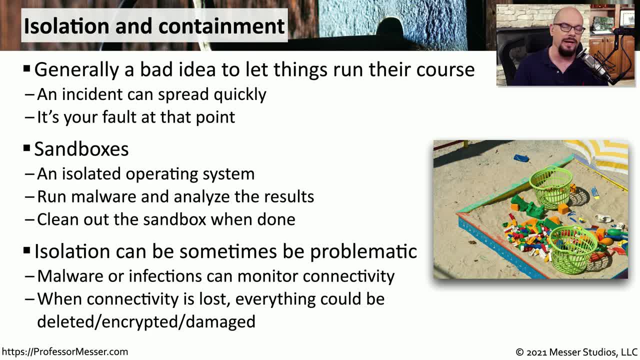 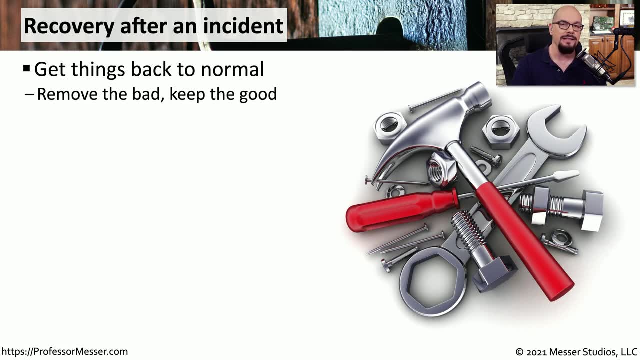 and it will perform differently. And if it's running in an open network And there's some malware that recognizes when you lose connectivity to the internet. So when you isolate that system it begins deleting files or damaging the operating system Once we've identified that an incident has occurred. 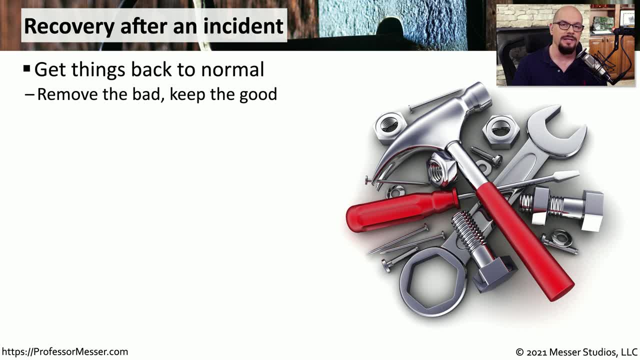 and we've identified where malware might be on a system, it's time to recover that system. We would first need to eradicate this malware and remove it from that system. Sometimes This involves completely deleting everything on the system and recovering from a known good backup. 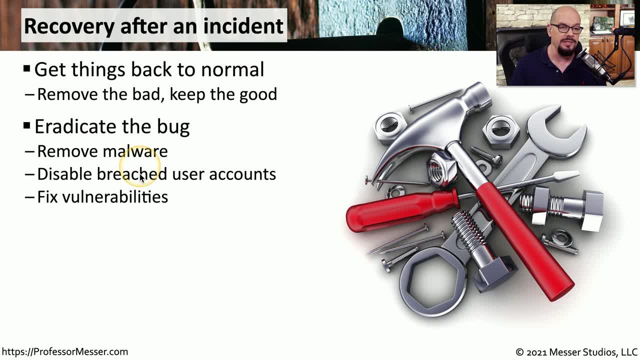 or a known good image, Or we may want to recover the system and then fix the vulnerabilities that caused this incident to occur in the first place. This is why it's always important to have a backup, so that you can restore this system very quickly. 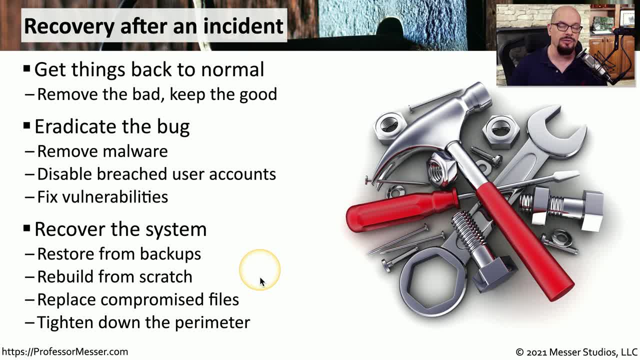 If you don't have a backup, then you'll need to rebuild the entire system from scratch, And in some cases, you may have lost data because you don't have a backup. In either of those situations, you'll want to be sure that you have rebuilt the system. 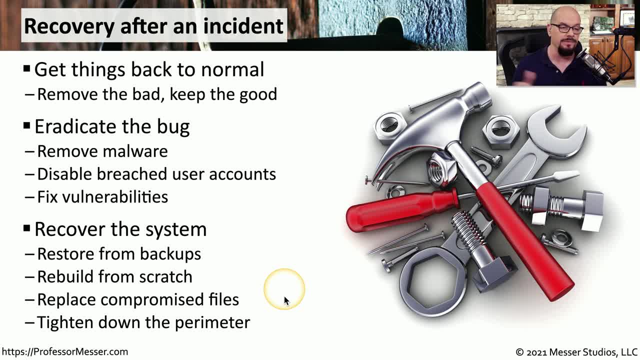 and that you have then repaired the system to close any of those vulnerabilities. And, lastly, you'll want to lock down the perimeter of the network so that you can stop the attack before it gets into your private network. On large networks, the reconstitution process. 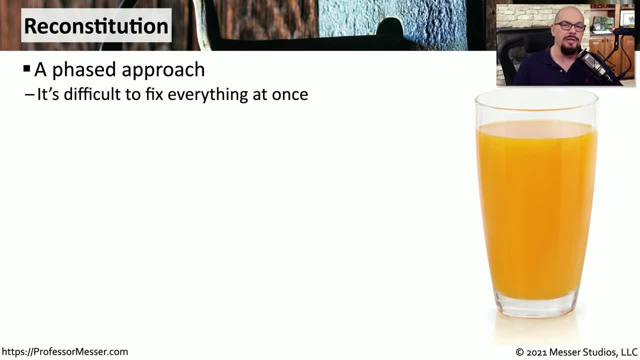 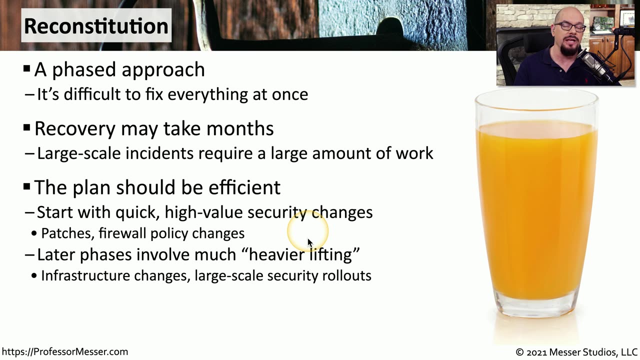 can be very difficult and very time consuming. You want to be sure that you have cleaned every system that could have been touched by this malware or this security incident, and this might take months of work to be able to recover everything on the network. This usually starts with making high value changes. 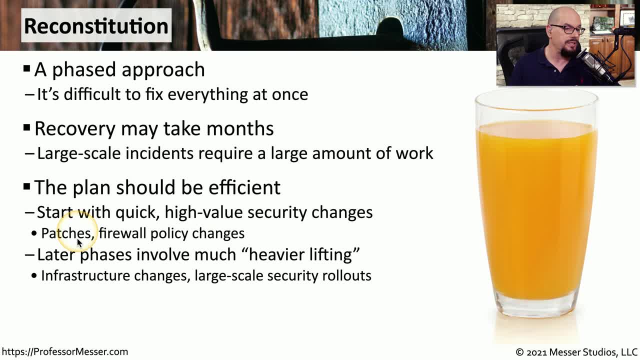 and making changes. that can be done very quickly. So we may want to send patches out to our systems or modify the firewall to prevent a certain type of traffic from entering your network. Then you can look at a much larger response across the entire infrastructure and begin. 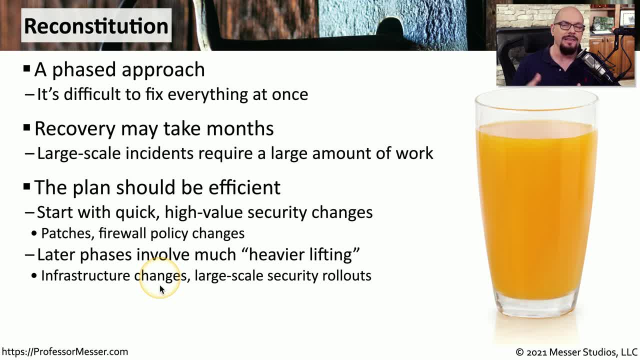 looking at changes in how the network is designed, look at the operating systems that may be used for a particular project and perhaps roll out additional systems and additional security controls, so you can prevent these types of incidents from occurring again. And once the incident is over, we 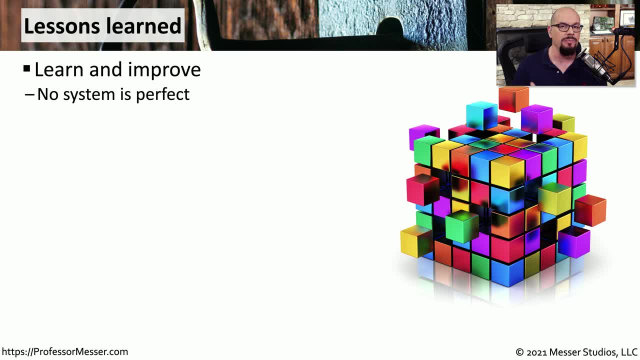 can take a step back and look at what processes worked and what processes didn't work during our incident response. We might want to have a post-incident meeting where everyone attends to talk about what occurred during the process, and we want to be sure we do this as quickly as possible.